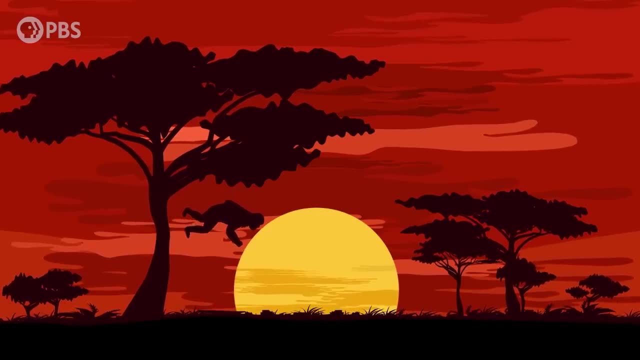 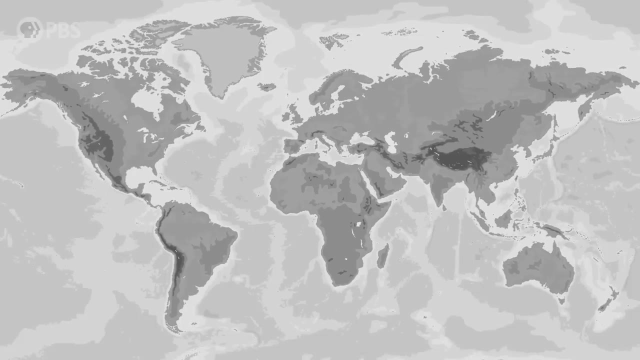 And it turns out that Lucy's fall might be a question that's as much about how our ancestors lived as it is about how she died. In 1974, when Lucy was first discovered in what's now Ethiopia, it was immediately clear that she was a big deal. 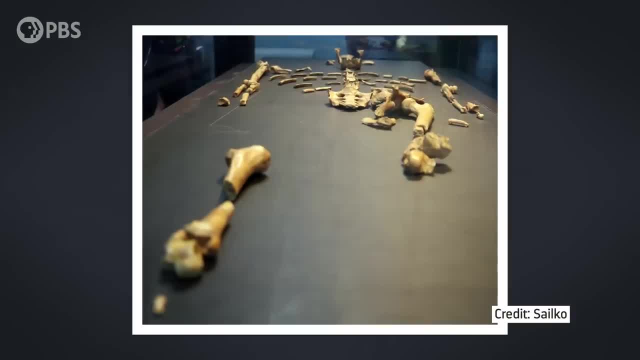 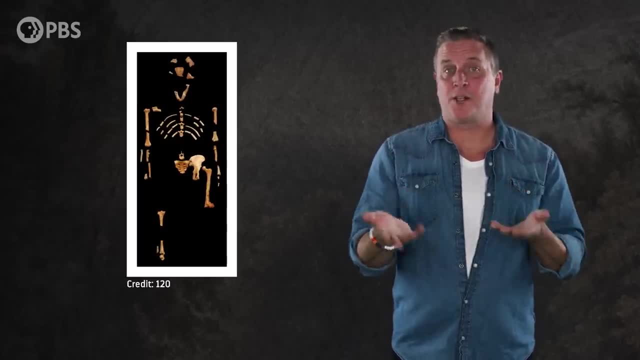 From the arid soils, scientists recovered a lot of her fossils, including fragments of her jaw, spine, ribs, pelvis, arms and legs. Her skeleton was about 40% complete, which meant that she contained tons of information. In contrast, previous discoveries from Africa were often limited to skulls, jaws and teeth. 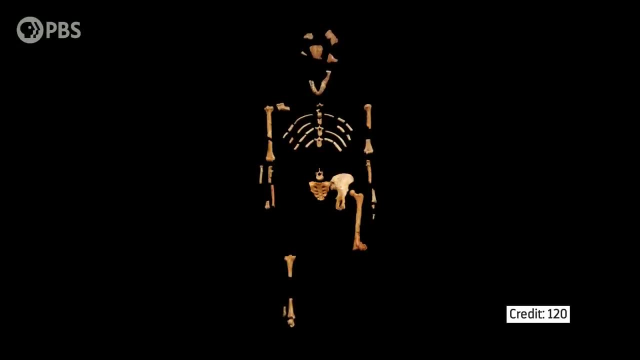 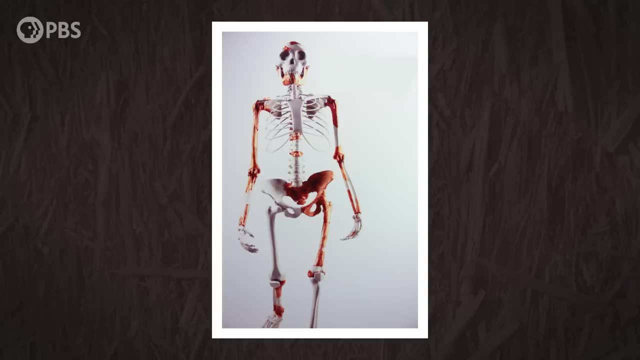 Also, she was really old. By dating the volcanic layers surrounding her fossils, scientists found that Lucy had been deposited just after 3.18 million years ago. This made her the oldest fossil human ancestor found at the time, And this meant that she could answer questions about the evolution of some of our most unique adaptations. 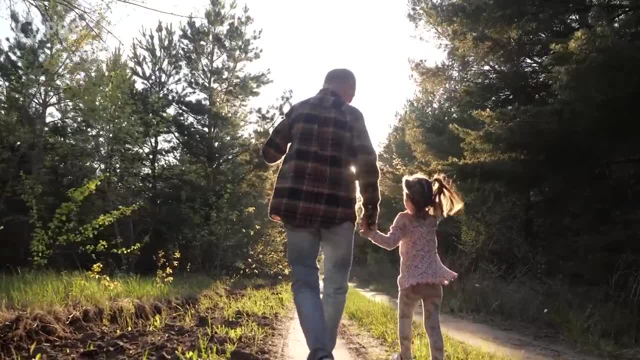 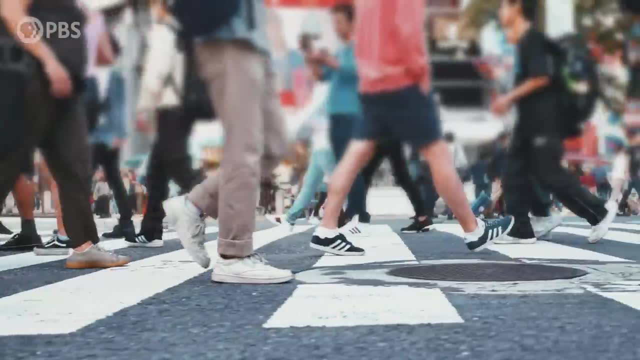 For example, in what order did our ancestors acquire each of the traits that make up our unique suite of features today, Like? did we evolve a big brain first, Or the ability to walk upright on two legs? Probably the biggest thing Lucy revealed is that bipedalism had already evolved by 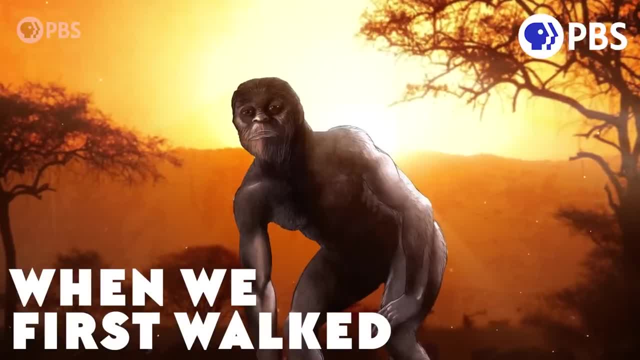 the time her species appeared- a topic we covered in another Aeons episode called When We First Walked. The shape of her pelvis, as well as the inward angle of her femur and some other features suggested that she was able to walk upright on two legs, and the shape of her pelvis, as well as the inward angle of her femur and some other features, suggested that she would walk upright on two legs. 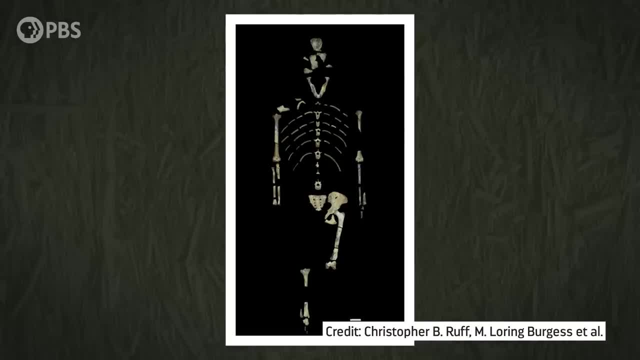 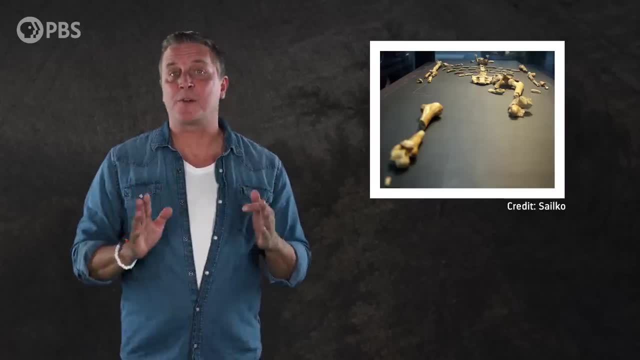 was already an obligate biped. She had to get around on two legs, not four. So the combination of Lucy's completeness, her old age and the insight she provided into our evolutionary history were the major factors that made her famous. Of course, it didn't hurt that she had a catchy nickname. Borrowed from the Beatles song Lucy in the Sky with Diamonds. the name was given to her the night of her discovery, when the team was celebrating, and that song came on. But since Lucy was uncovered in the 1970s, her story has only gotten more interesting. 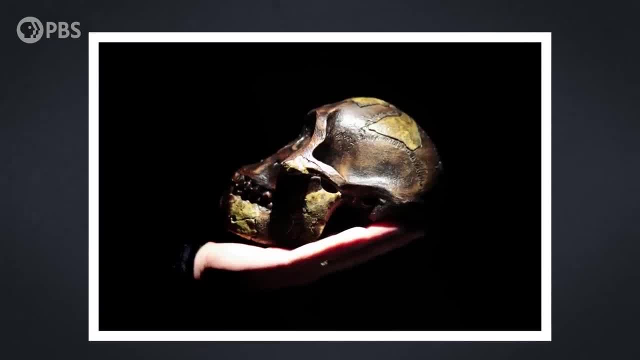 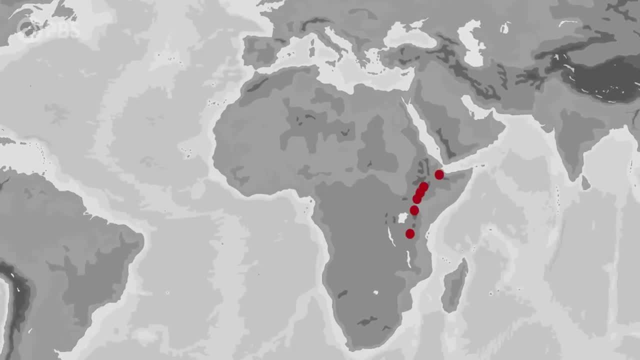 Scientists have continued studying her for decades and they've found more than 400 additional specimens belonging to her species, Australopithecus afarensis. These come from across Ethiopia, Kenya and Tanzania and date from 3.7 to 3 million years. 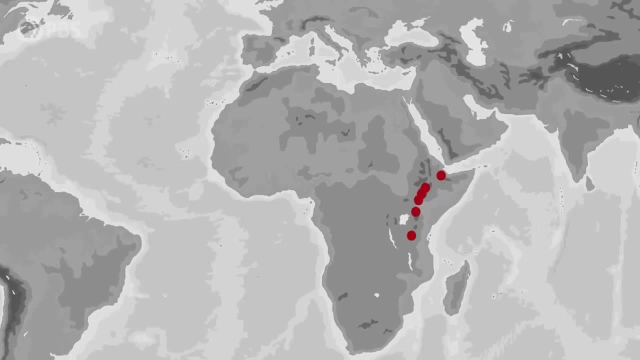 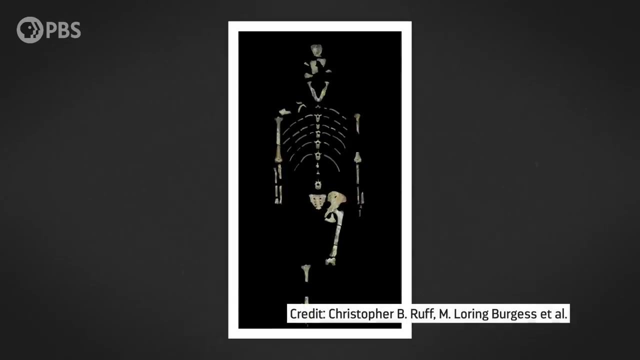 ago. This makes Australopithecus afarensis one of the longest-existing species of early human ancestors. But even after decades of research, we still haven't learned all there is to know about Lucy. In 2015,, a group of scientists became interested in the amount of damage they could see on 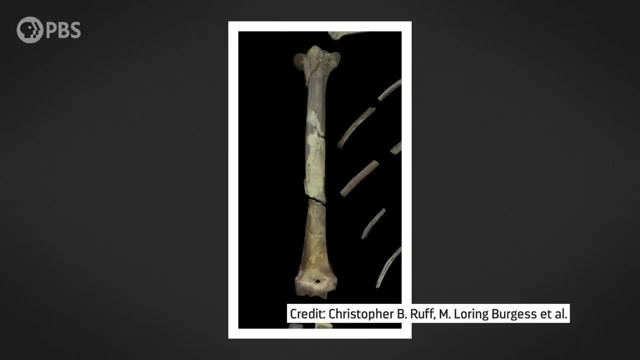 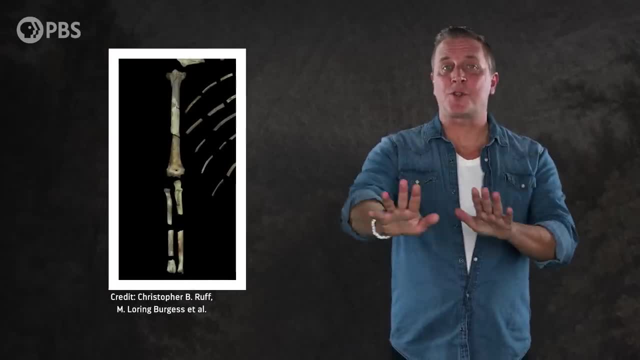 her fossilized bones, Lucy appeared to have a lot of fractures. Based on the pattern, they concluded that a fall from a tall tree had caused the breaks. Their interpretation of the fractures was that Lucy had stretched her hands out in front of her to try to stop her fall, breaking her hands, wrists, arms, shoulders and jaw in. 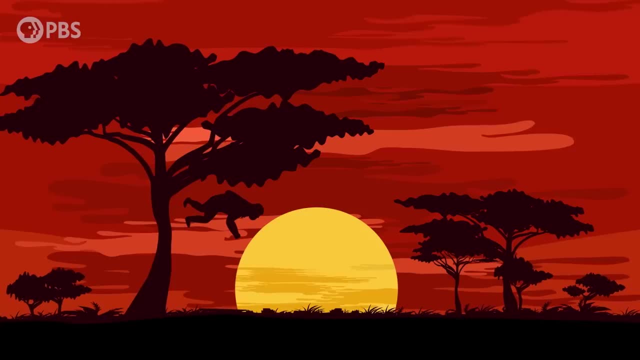 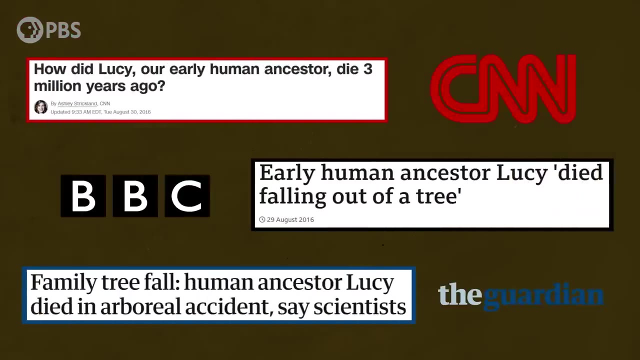 the process. Basically, she was a wreck. It was an astonishing idea, one that allowed us to vividly imagine what might have been her final moments. But while the idea that Lucy fell made headlines all over the world, it was received a bit. 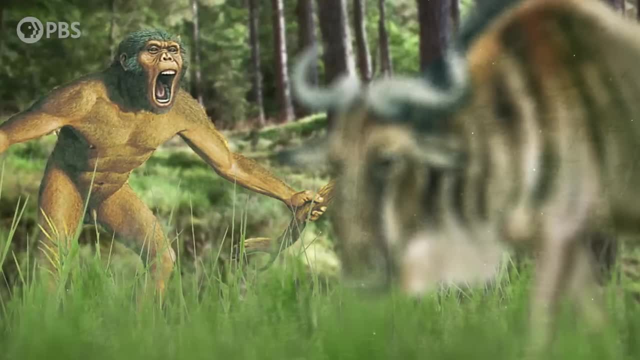 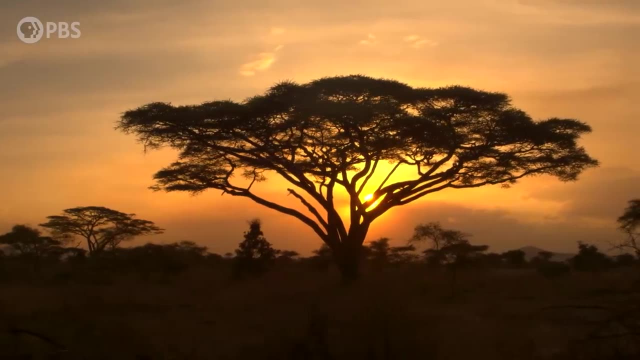 more skeptically across the scientific community, Because it fueled a debate that, like Lucy herself, had been around for decades. Did life in the trees remain important to Australopithecus afarensis even after they found their footing on the ground? 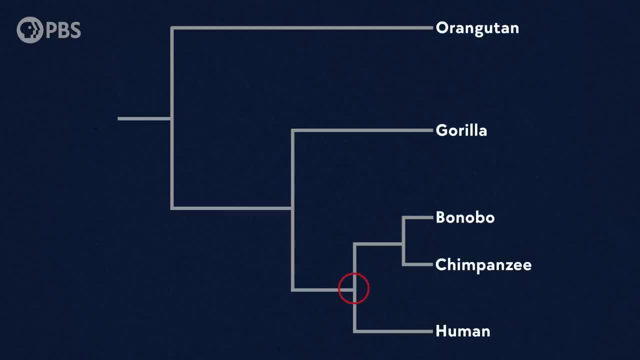 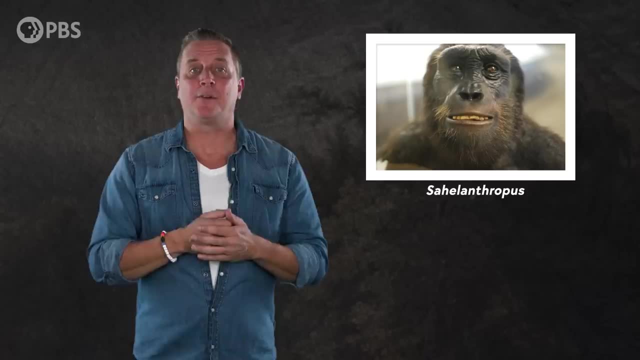 Now we know that, before our lineage split off from the one that led to chimpanzees, our shared ancestors were up in the trees. After that split, the members of our branch of the family tree transitioned to life on the ground, potentially starting around 6 or 7 million years ago. 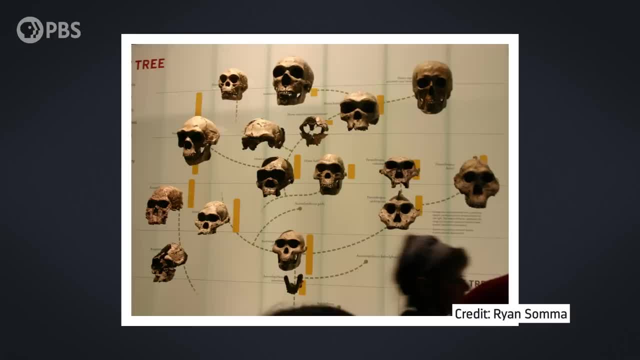 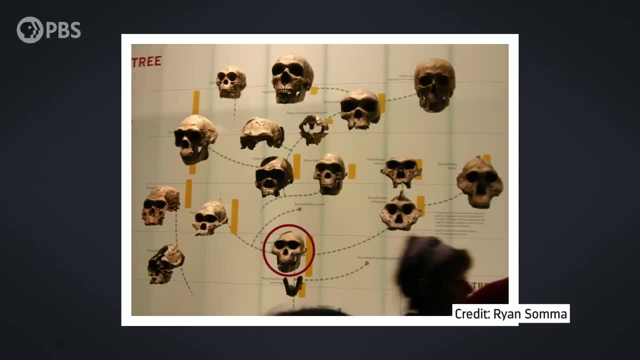 But the move down to the African forest floor didn't happen overnight. There were likely many different stages in the transition And because of where Lucy sits in the family tree, her species potentially is a key piece of the puzzle. And since we can't go back in time and observe whether Lucy was hanging out on trees, we 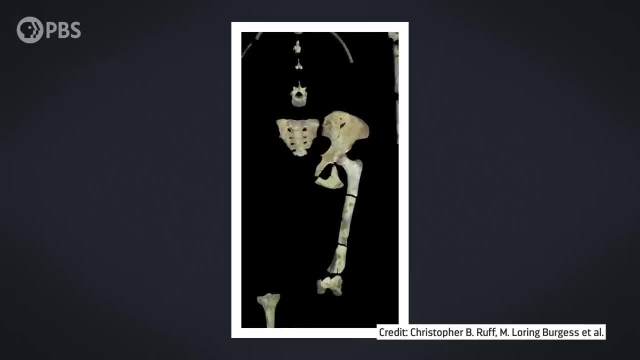 have to go on the skeletal evidence. We already know from her lower body, specifically her femur, that there's no question that Lucy and other members of her species were adapted to be skilled walkers. But when we look at their upper bodies the picture starts to get interesting. 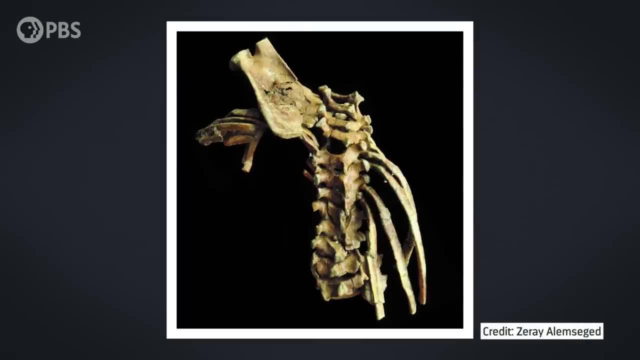 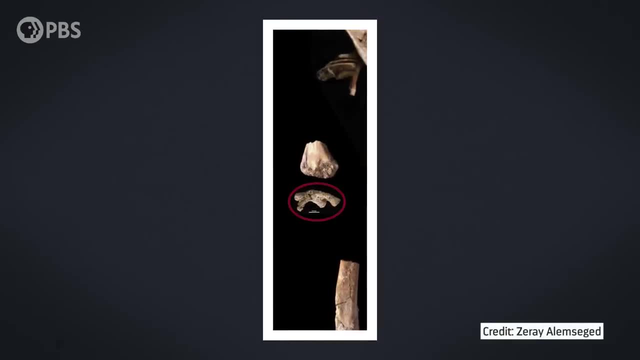 A shoulder blade preserved from a juvenile of her species nicknamed Lucy's Baby looked more like a tree climber than a permanent tree climber, And the slightly curved finger bones seen in her species are well-adapted for grasping branches. So Australopithecus afarensis had some adaptations from moving through the trees. 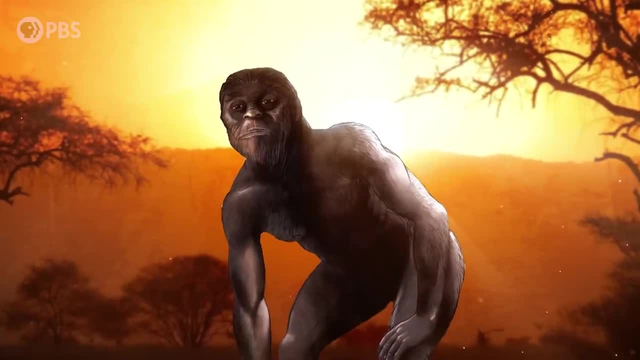 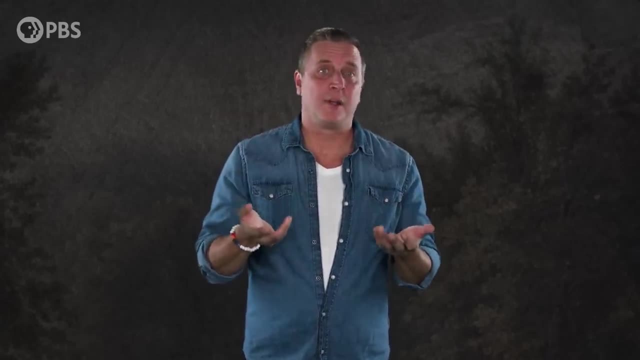 But did they actually use them? Some scientists think that these traits in Australopithecus are just a useless evolutionary holdover. See, natural selection really only modifies what's important at that time. Other stuff sometimes just gets left as is sticking around long after losing its evolutionary. 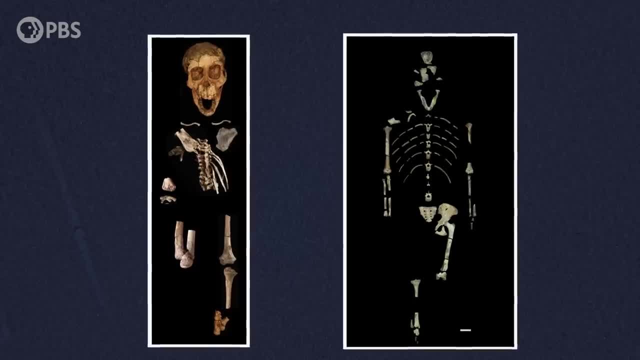 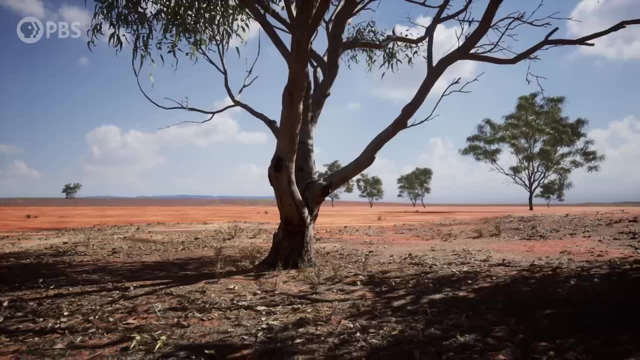 purpose, And this brings up an important distinction. Does the skeletal evidence point to things that a hominin's body could physically do, Or is it pointing to a thing that hominins actually did? There might have been some advantages to being a good tree climber, even after becoming a 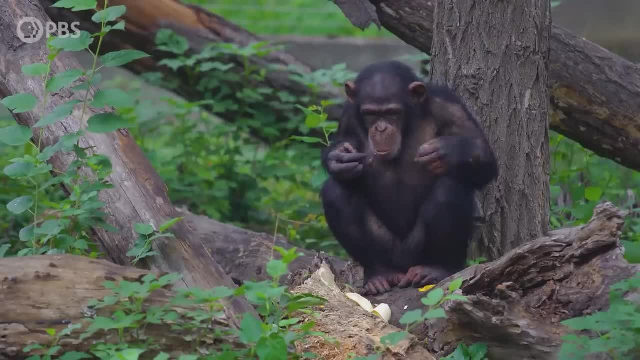 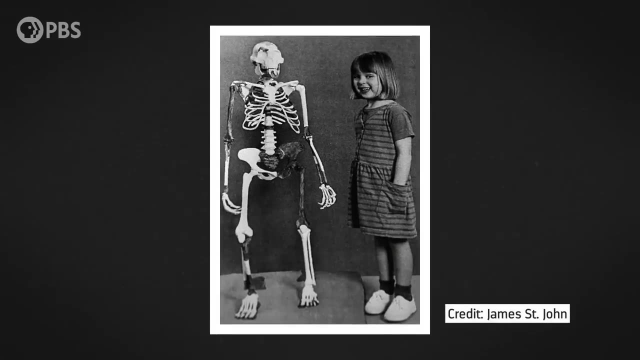 good walker. For example, some other ground-dwelling apes, like chimpanzees, often build nests and tree canopies to sleep. This strategy would have worked well for hominins like Lucy. She was small, only about a meter tall, and not particularly fast. 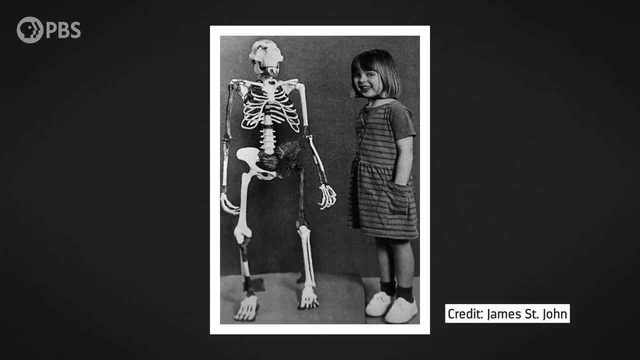 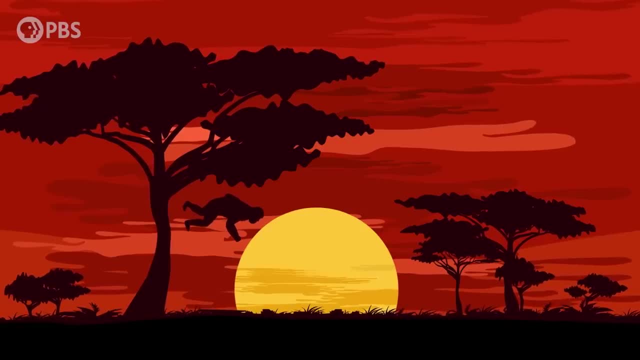 A prime candidate to be preyed upon by big cats and other fierce predators, But behaviors like nest building and canopy sleeping don't really work for her. So we'll have to wait and see. And this is where Lucy's fall comes in. 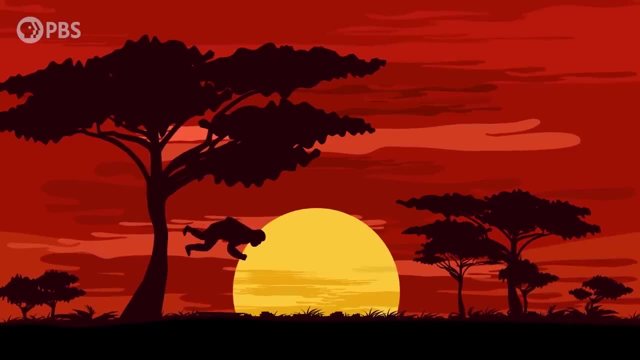 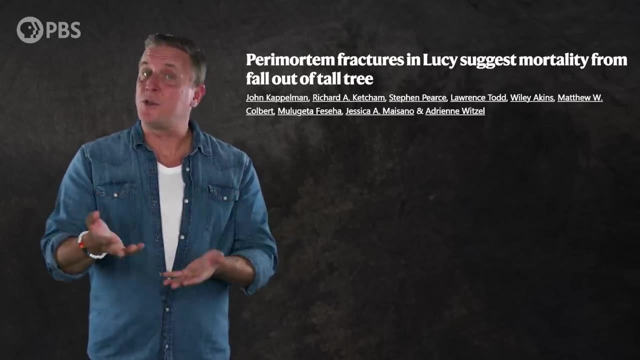 It offered a potential new type of evidence that theoretically showed what Lucy actually did. By arguing that she fell from a tree, the researchers were suggesting that she was essentially caught in the act of being in trees, And while broken bones that might have been caused by falls have been proposed for other 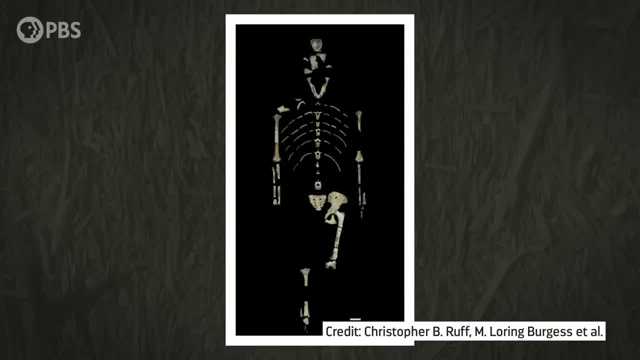 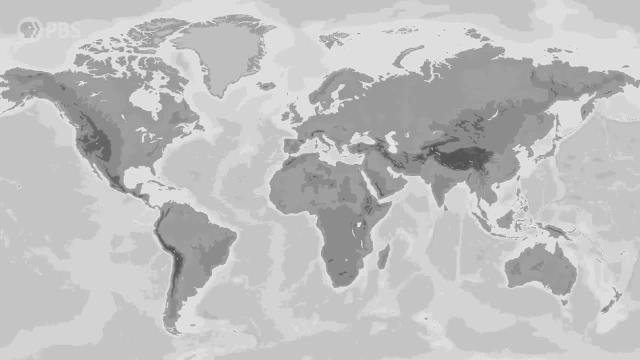 hominins. there was one major problem in this particular case: Their fracture patterns weren't unique to Lucy. When the 2016 study that put forward the fall idea first appeared, researchers working at her discovery site, a place called Hadar, quickly objected. 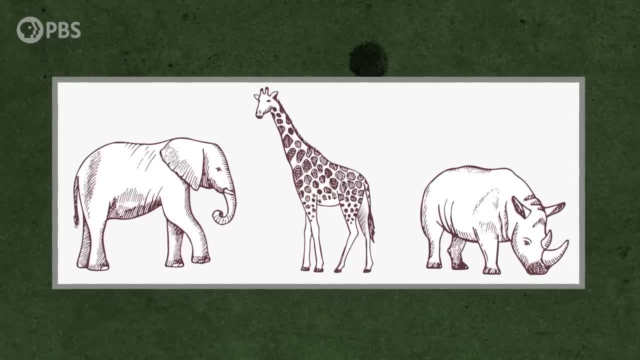 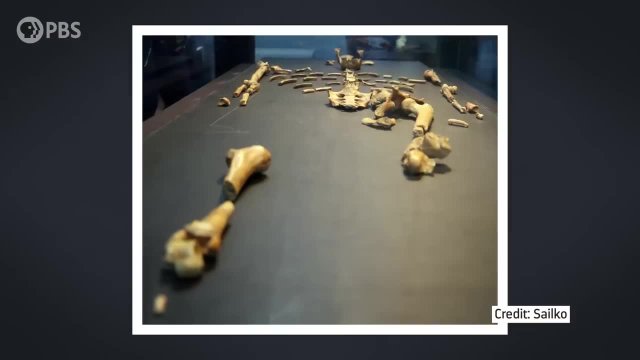 They said that similar fractures were prevalent on the bones of other animals like elephants, giraffes and rhinos, found throughout the site, not just on Lucy. Lucy's discoverers pointed out that it was more likely that the damage was produced by 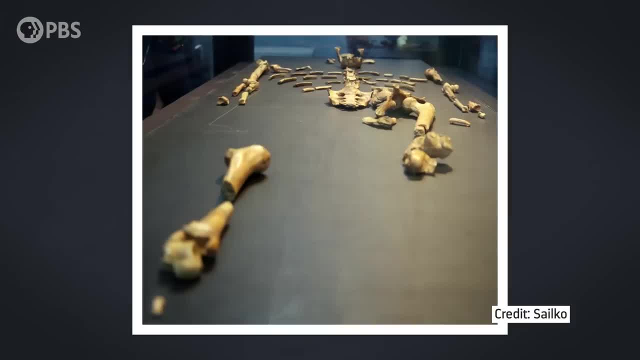 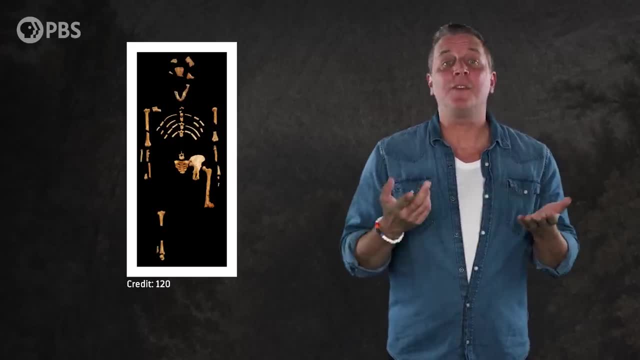 fossilization processes resulting from millions of years in the ground. During that time, their bones were probably exposed to water, crushing events, pressure from the sedimentary layers above erosion and even plate tectonics. This type of damage better explains why these fractures appeared across species and why. 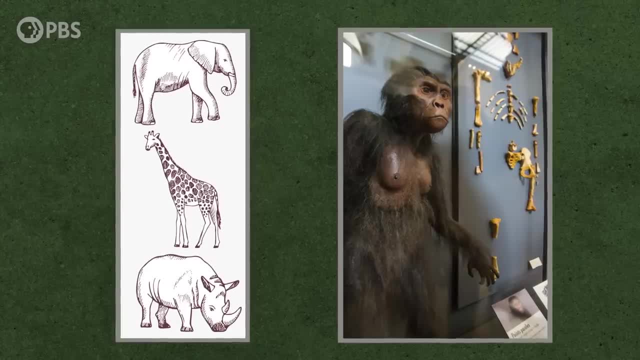 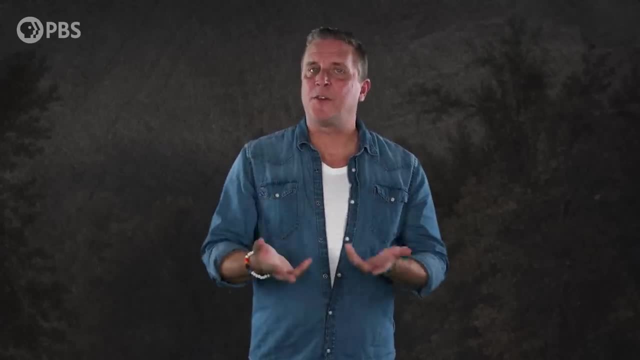 they were so common. But it wasn't just Lucy. There were other species at this single location Because, as one researcher pointed out, rhinos weren't exactly falling out of four-story high trees. So while Lucy's fall was possible, the scientists hypothesizing it didn't consider all the 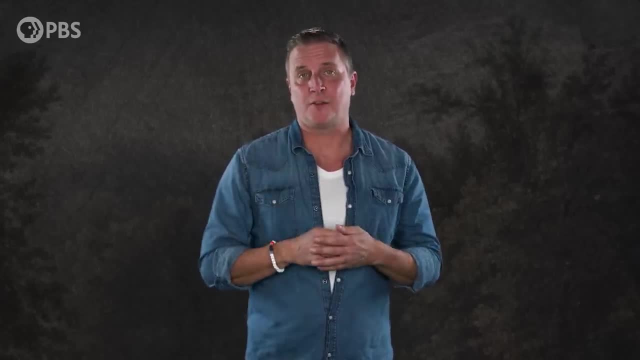 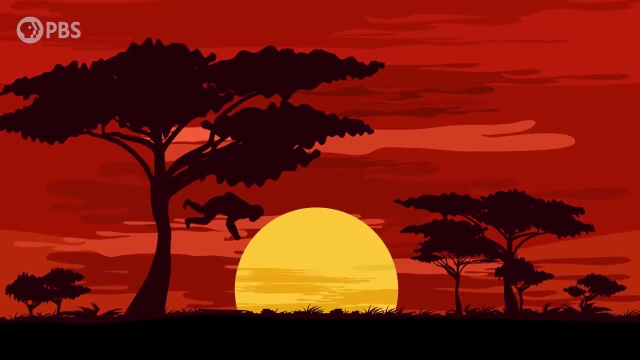 other explanations for these kinds of fractures, which is a must in science, And the question of whether her species still spent time in the trees, or how much time they spent there, is still open. So, while the fall hypothesis kind of lost its footing, what the study really shows is: 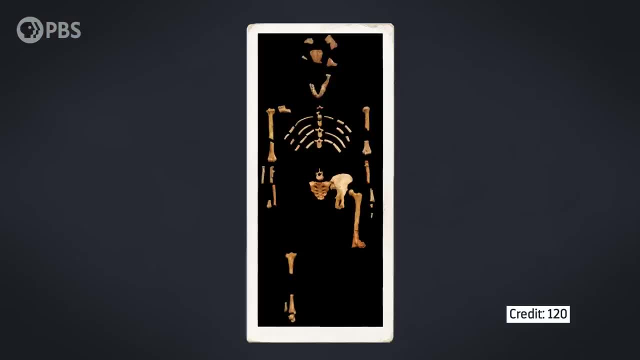 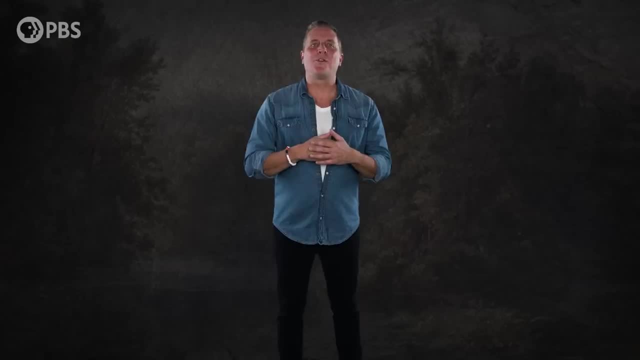 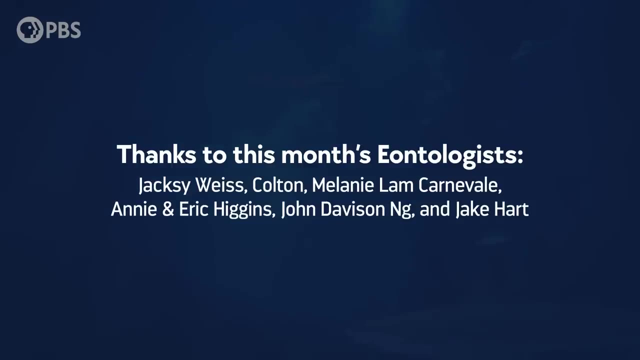 that Lucy's bones still have things to teach us, And even after decades of research…. We're falling for this month's Eontologists: Jack C Weiss, Colton, Melanie Lamb, Carnevale Annie and Eric Higgins, John Davison, Ng and. 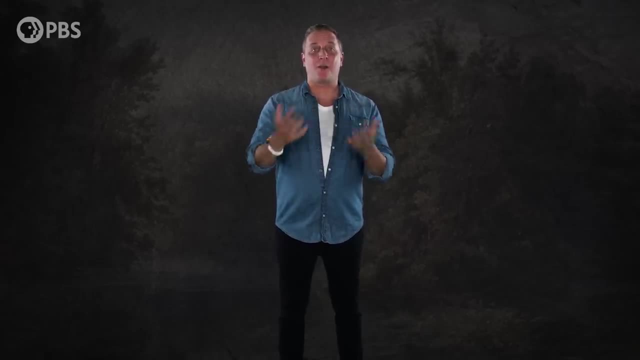 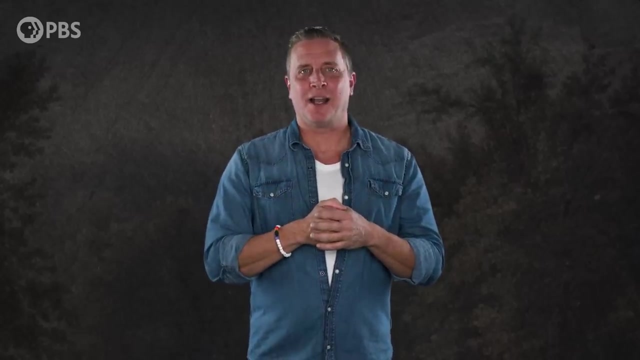 Jake Hart. Become an Eonite at patreoncom. slash eons and you can get fun perks like submitting a joke for us to read, Like this one from Cassie W: Where did the female Dromusaurid live? I don't know, but Alaska.